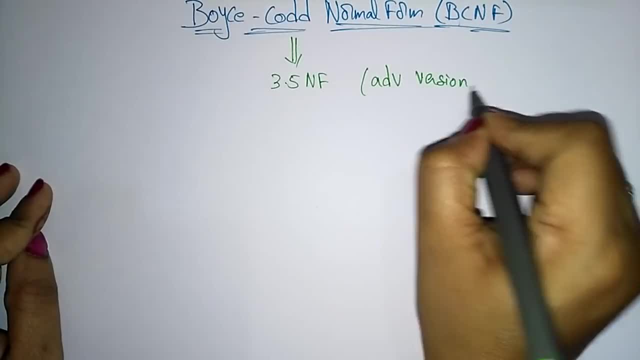 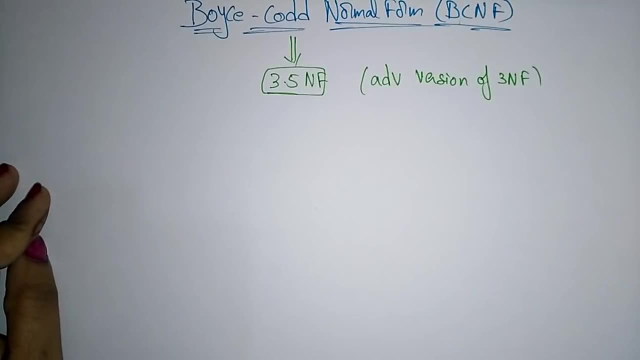 customized advanced version of 3NF. So that is why we call it as a 3.5 normal form. So the another name for this BCNF is 3.5 normal form. So what are the conditions to follow for? 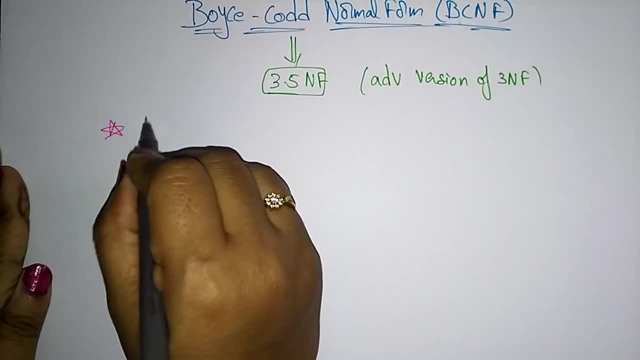 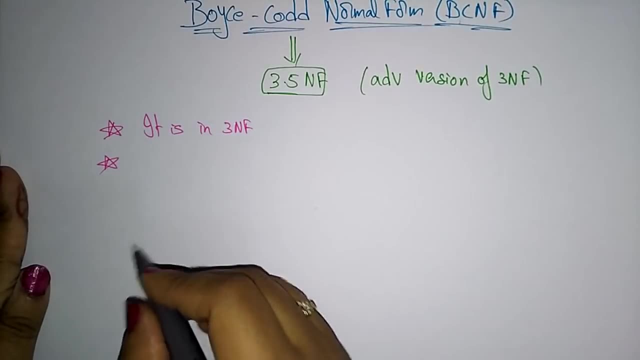 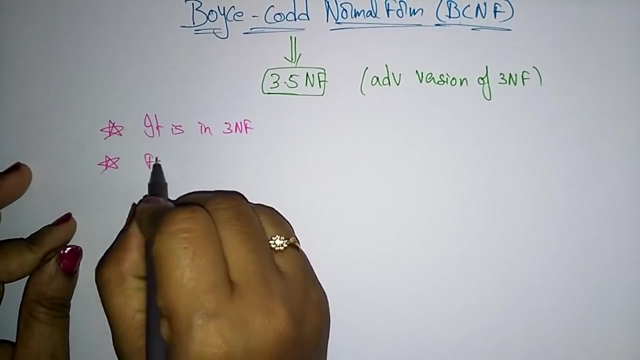 BCNF. So the first it should be. it is in 3rd normal form and next, whereas in 3NF the first it should be in 2NF, after that there is no transitive dependency in 3NF, but here in BCNF it is in first, it should be in 3NF, Next for every. 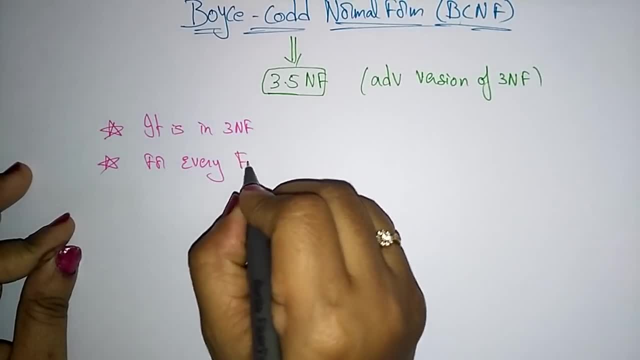 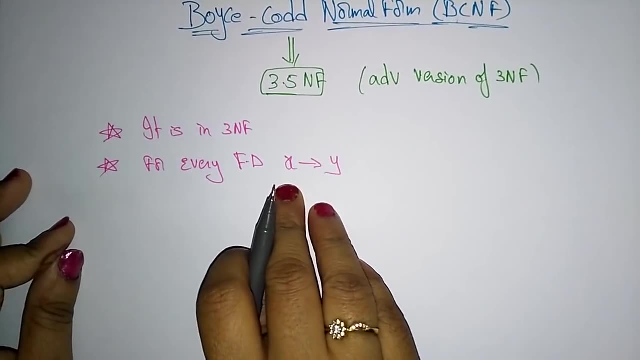 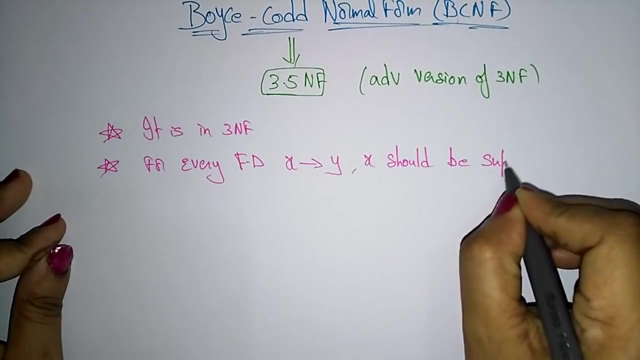 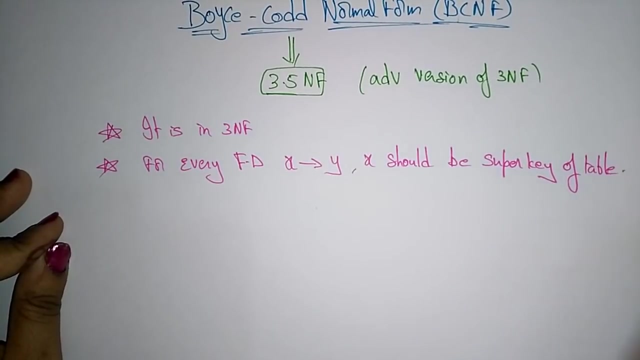 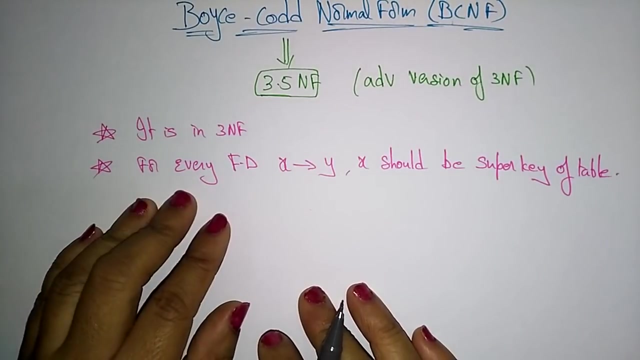 for every functionally dependency. that is, x determines y means y is functionally dependent on x. here x should be super key of a table. So this is a main point. you have to be remember that. so whereas in 3NF there is no transitive dependency, and whereas in BCNF for every 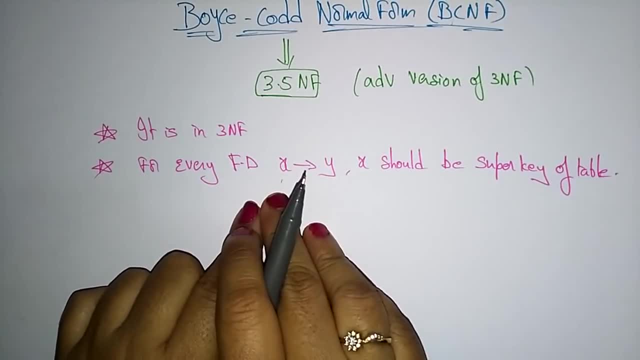 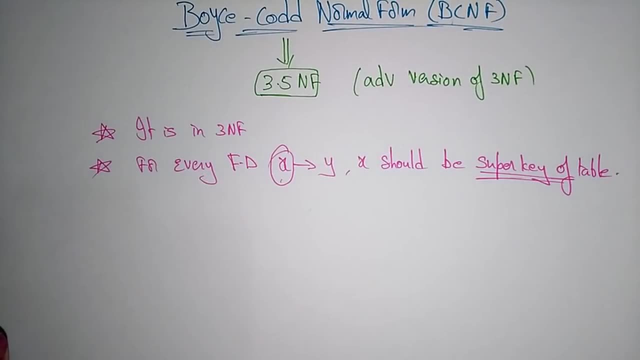 functionally dependency, that is, x determines y, means y depends upon x. this x should be super key of a table. So you have to be in 3NF, So this is a main point. you have to be remember that be checked whether the key attribute is a super key or not. okay, so let me take an example for this. 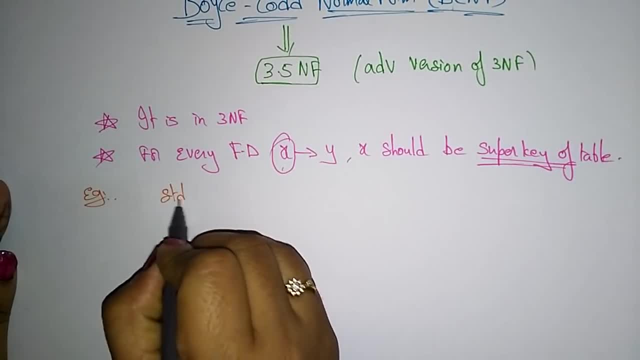 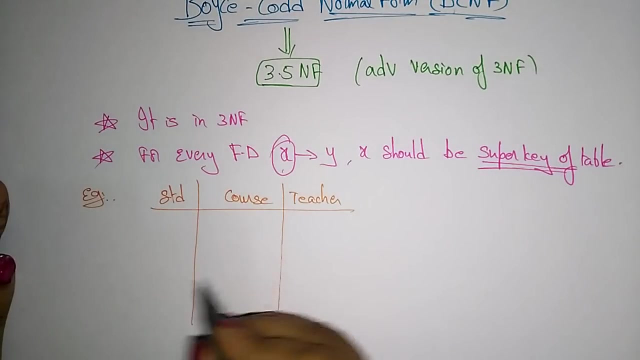 boys bcnf. so this is a student table, student course and the teacher who teaches that course? okay, so let me take this table. so here in this table, the fields for this. or let me take the fields. suppose the pinky pinky is doing the course dbms. 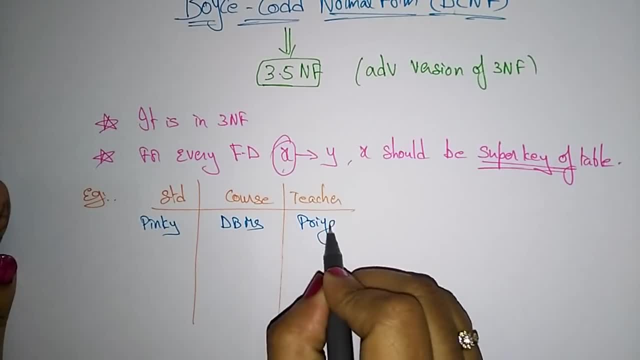 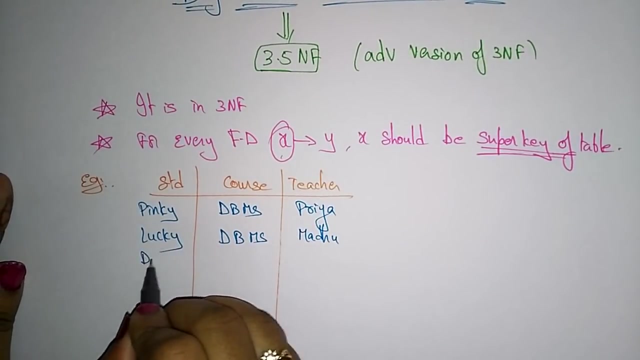 and the teacher is priya, and next lucky. so lucky is also dealing with the course starting the course dbms, and the related teacher is. but here for lucky, the another teacher that is a madhu dipu coa and who teaches uh bhanu, next bhanu, she also learning the course coa, the same teacher, uh, so sorry, here the teacher. 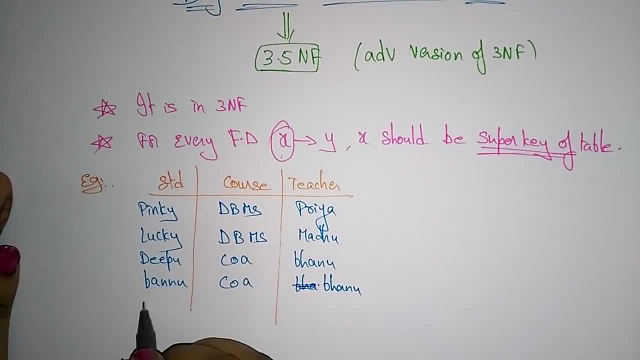 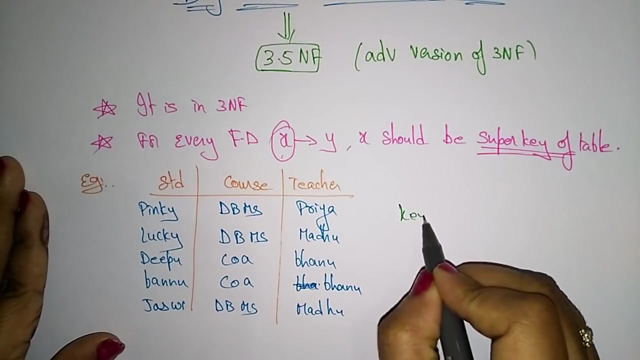 should be the same teacher. let's take bhanu and jasvi dbms. so here, only two courses are there, uh, and the teachers are different. teachers are teaching the different course, i mean the same courses, this course are teaching different teachers. so here so much of written-in data. is there multiple data is there? so, uh, in this the key attributes, or let 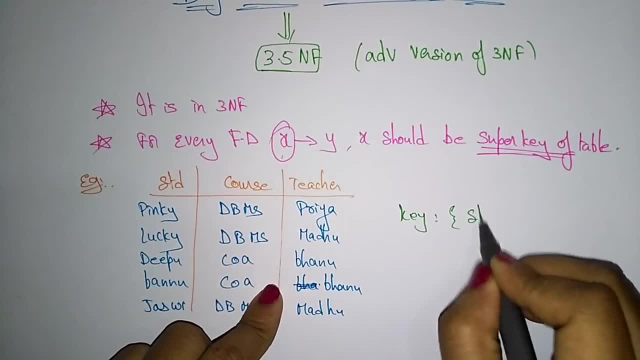 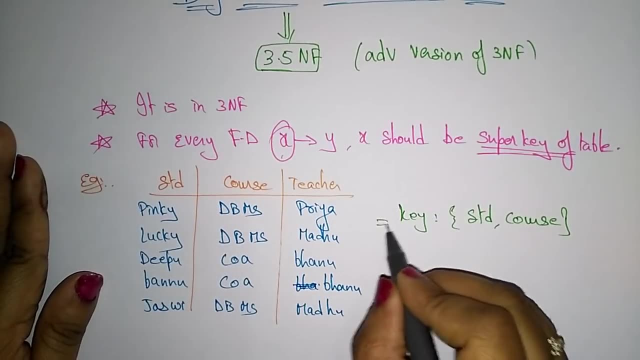 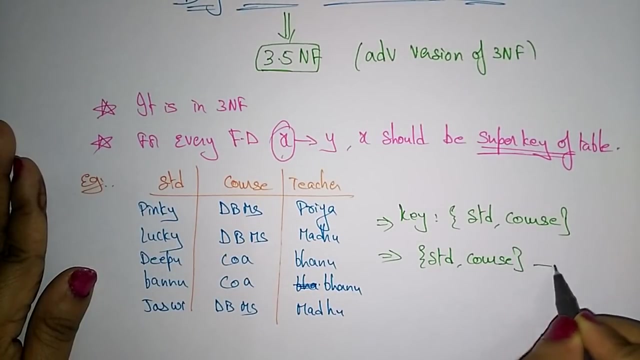 me take this. keys in this table is: let's take student and course, both of the keys. student and course, both are the keys and the functionally dependency is. the student course determines the teacher, because teacher is a non-key attribute, the non-key attributes, communities are sacred to all we are. nature small is still. we are creating some. 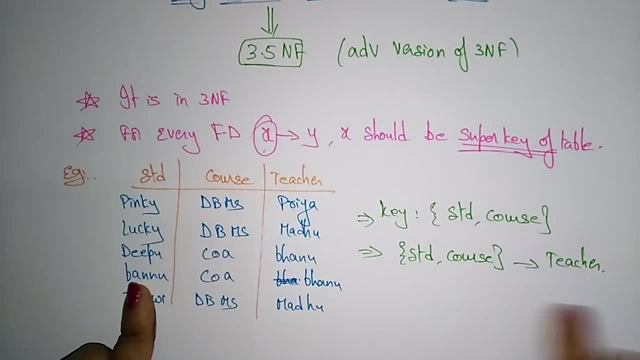 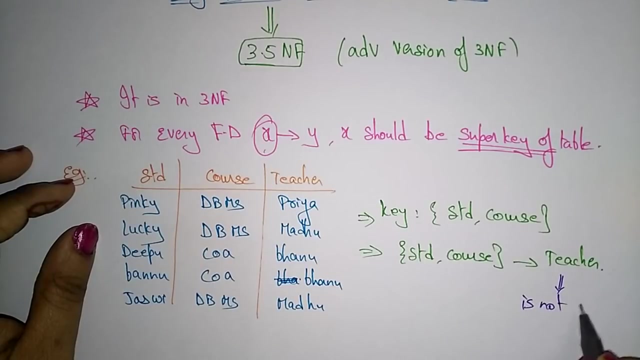 attribute is fully functionally dependent on the key attributes. So the functional dependency here is: teacher is a non-key attribute and depends upon the student and course. So what is the problem here? So the problem here is: teacher is not a super key. Okay, here the teacher is not super key. 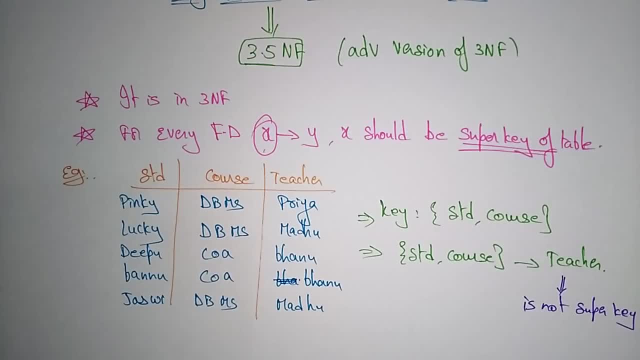 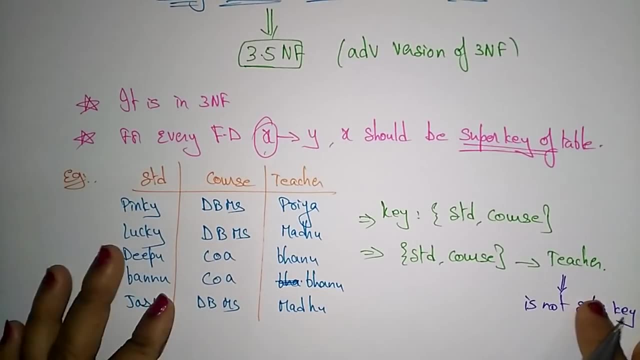 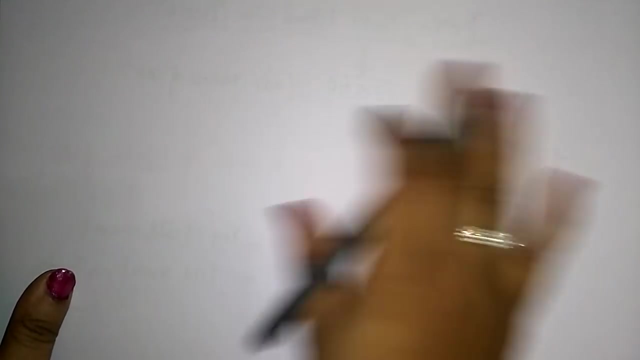 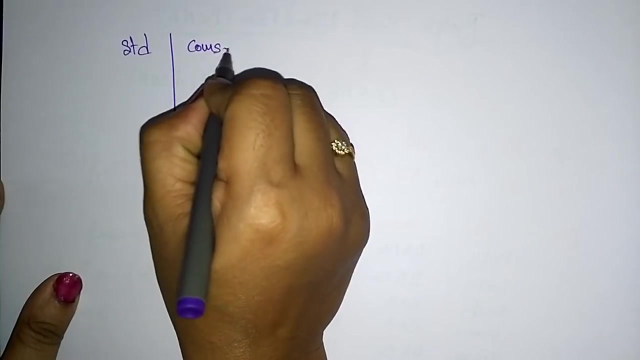 but determines the course. Okay so, teacher is not a super key, but determines the course. So now let's convert this table into BCNF. So let us see, after decomposition, decomposing, what is the BCNF tables. Let's take, divided the table into two tables, student and the course is one table. 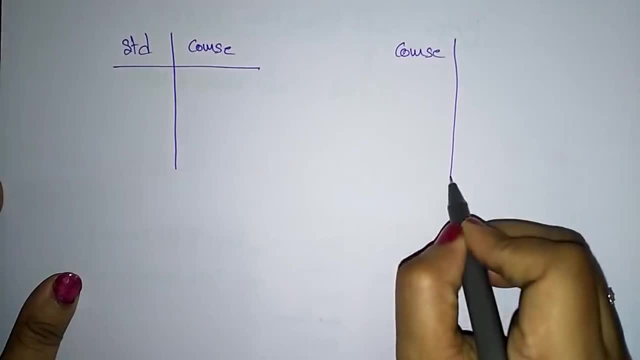 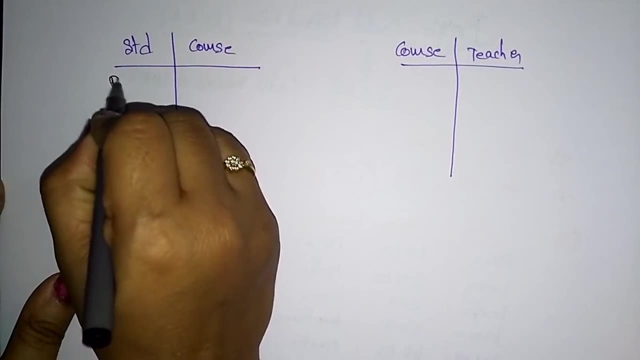 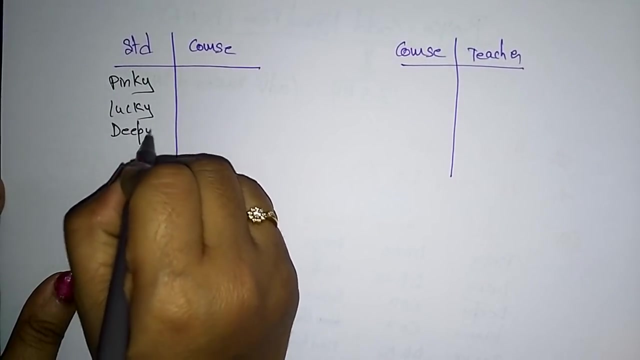 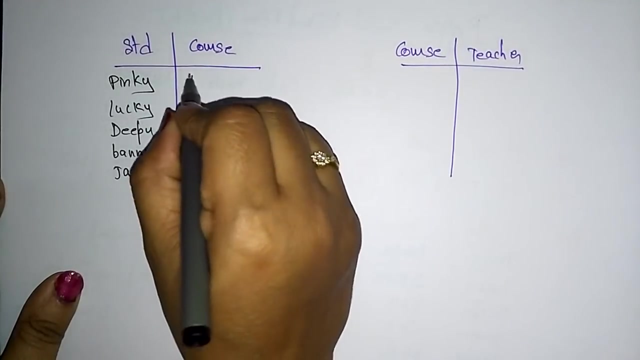 and here a course teacher is another table. So here a student, sir pinky here. so here a student, sir pinky. so here a student, sir pinky, Lucky, Deepu, Banno and Jasvi. So these are the student names and the related courses for those students. is Pinky is doing DBMS. 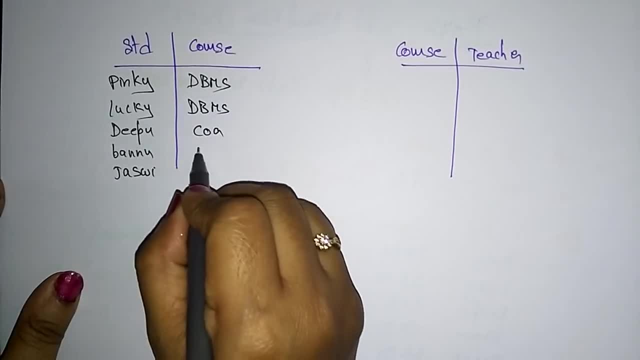 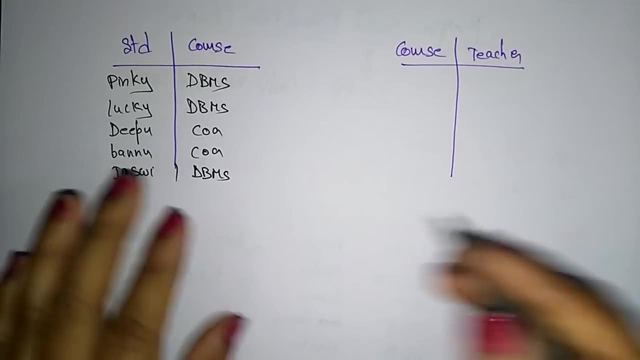 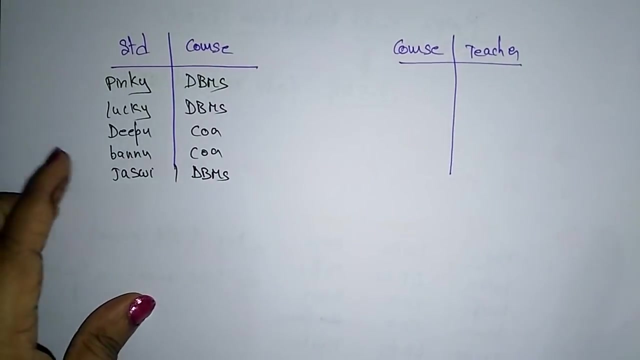 Lucky is also DBMS, COA and DBMS. So this is one table. Now coming to another table. So here the courses, or only the two courses, are there, But in these two courses, only for one, for these two courses, here a COA is teaching.